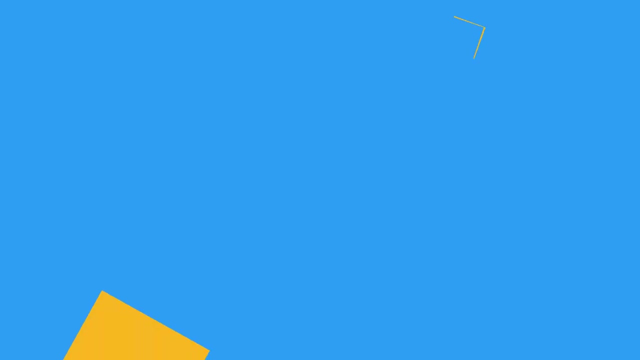 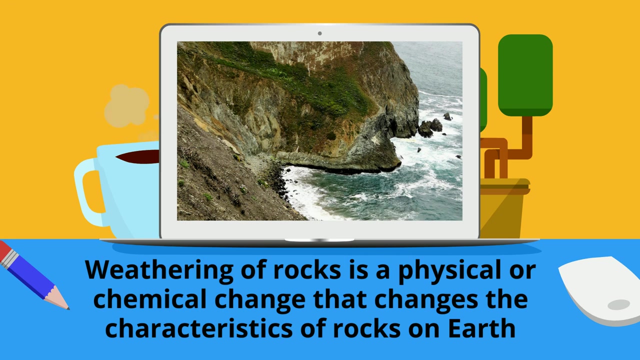 Welcome to MooMooMath in Science and Weathering. Weathering of rocks is a physical or chemical change that changes the characteristics of the rocks on earth. There are two major types: Physical weathering, which involves breaking rocks into smaller fragments, caused by 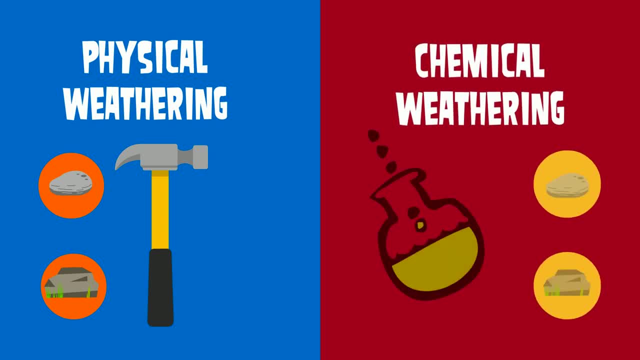 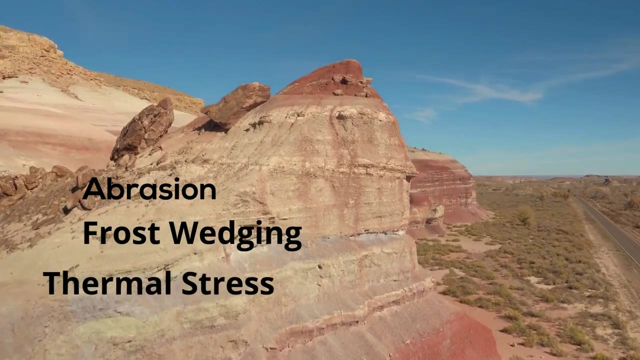 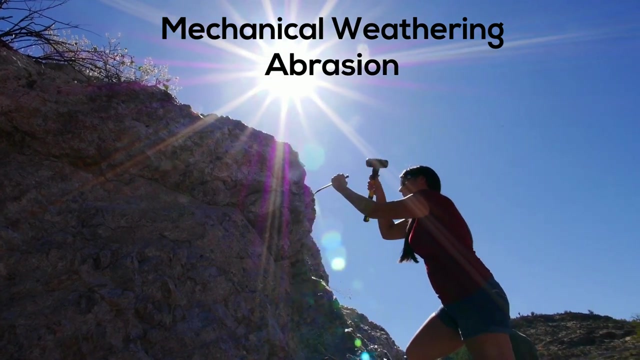 environmental factors And chemical weathering, which are changes that involve rocks being changed into new substances or minerals. chemically, Let's look at three major types of physical weathering: Abrasion, frost, wedging and thermal stress. Abrasion is mechanical scraping and can be caused by several factors. Basically, 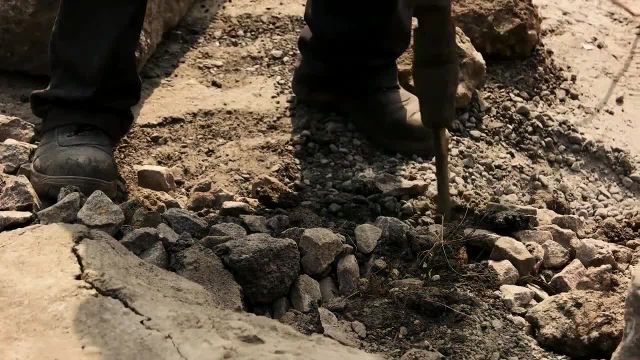 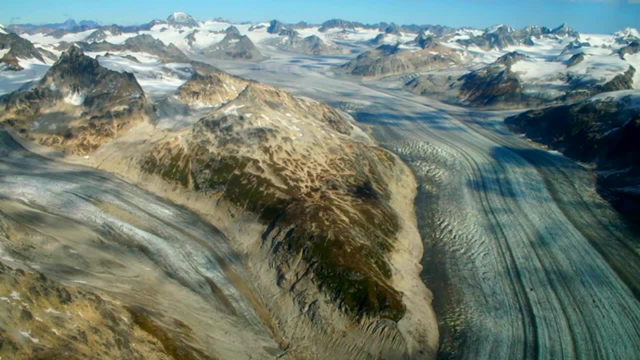 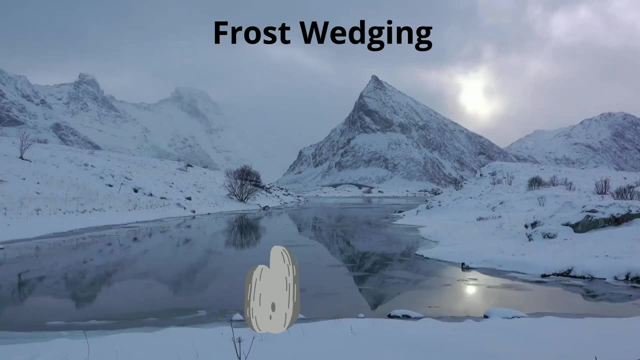 these factors just break the rock apart: Wind, water or waves, glaciers, gravity and even plants and animals. Frost wedging occurs as water expands, as it freezes, and this can cause the rock to break apart. Thermal stress is a type of weathering where 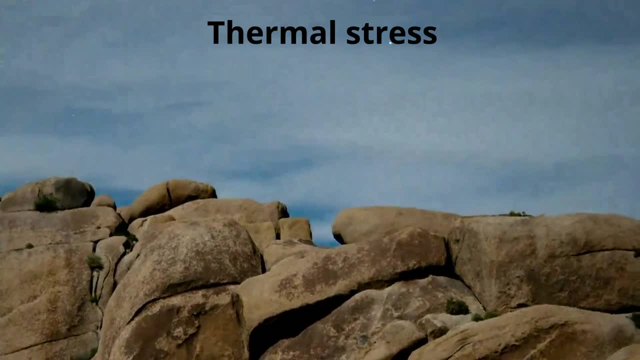 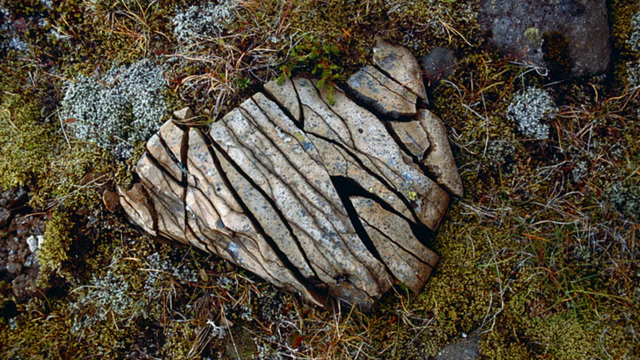 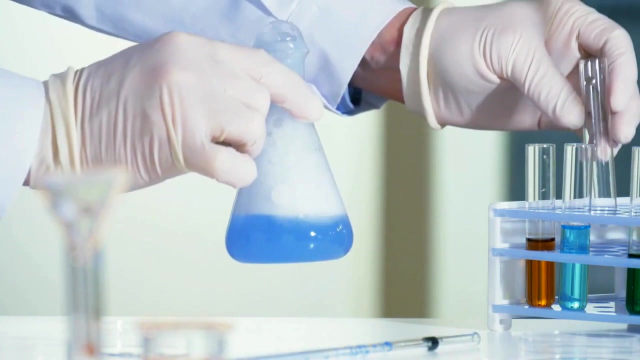 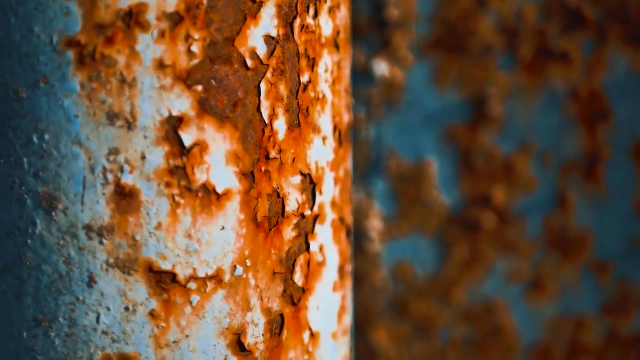 heat and changes in temperature cause the rocks to expand and contract and this can break the rock. Next let's look at chemical changes, of weathering. Remember a chemical change creates a new substance. There are three major types. First, oxidation occurs as oxygen combines with iron in the rock and creates a new compound. 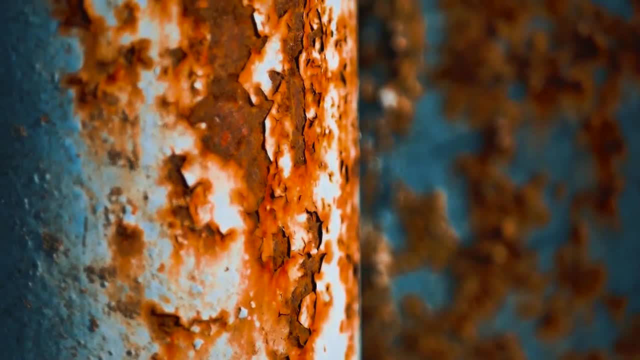 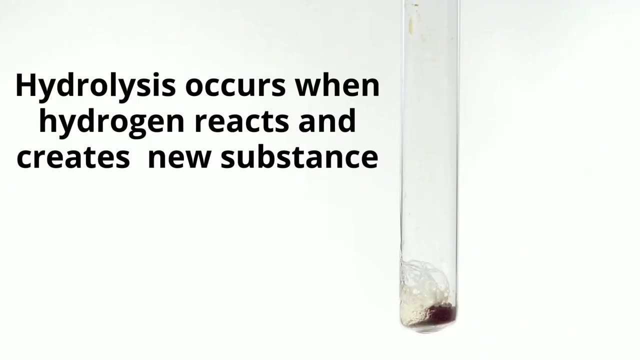 When iron reacts with oxygen, it forms iron oxide, commonly called rust, and this weakens the rock. Hydrolysis occurs when hydrogen or hydrate replaces the ion and creates a new substance. For example, hydrolysis causes field spar to turn into clay. 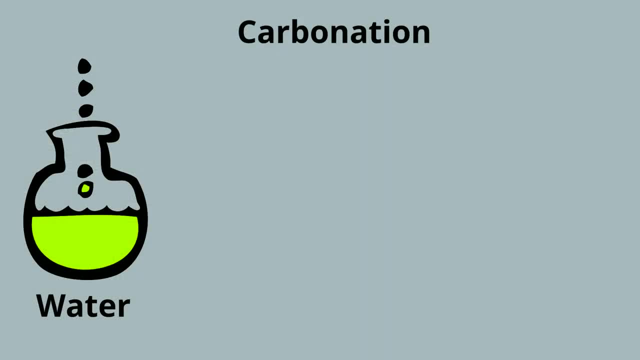 And finally, carbonation is the process of mixing water with carbon dioxide to make carbonic acid. This acid then breaks down and weakens the rock. Carbonation is the process of mixing water with carbon dioxide to make carbonic acid. This acid then breaks down and weakens the rock. 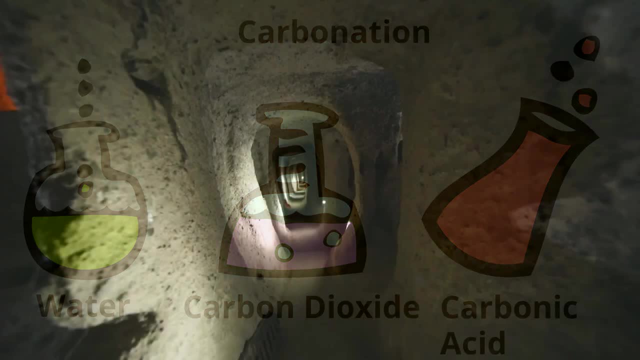 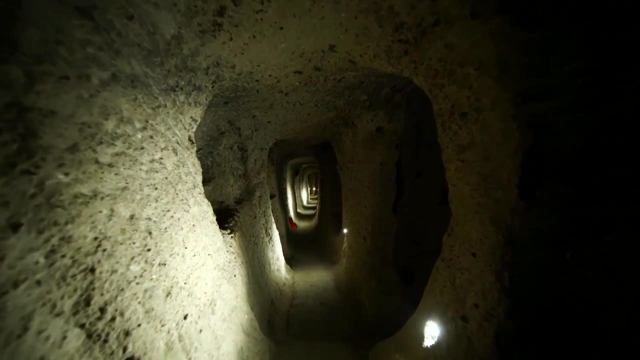 Caves may be formed by carbonation dissolving limestone. Caves may be formed by carbonation dissolving limestone. Rainwater picks up the carbon dioxide from the air and, as it percolates through the soil, slowly dissolves out the limestone.